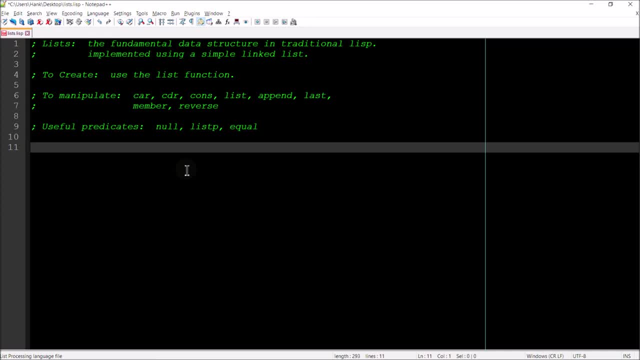 lists were, you know, the fundamental data structure, right? So later versions of Lisp added other things like trees and arrays and vectors, but way back when in the beginning, it was just lists, right? So a list in Lisp is implemented in memory using a version of a simple linked list and you're gonna see that. 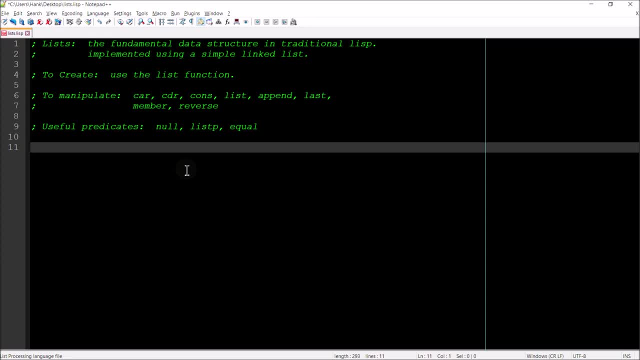 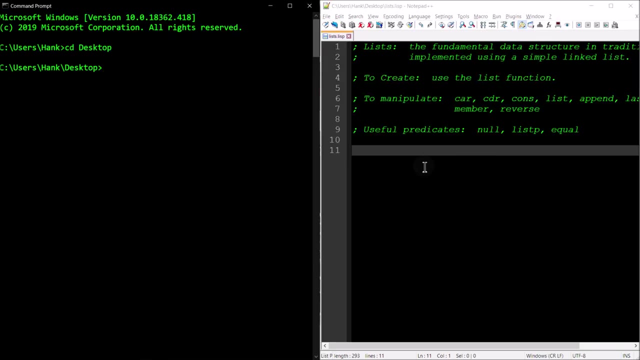 it's pretty easy to get started. So to get started with these things and to manipulate it, you know, you just have to use the appropriate functions, and I'm gonna also show you some useful predicates, right? So let's go ahead and get started. Okay, so a list can be made up of anything in Lisp. 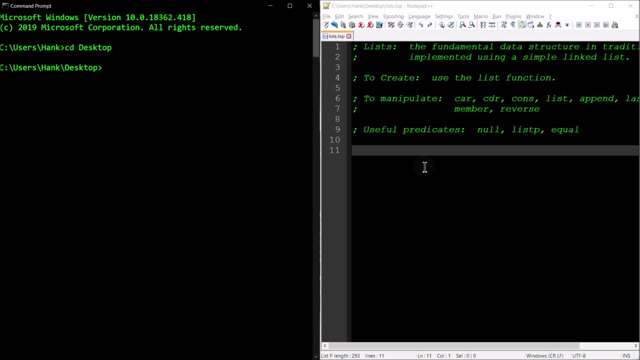 right, It can be made up of numbers: all different types of atoms. you know things like that, So let's go ahead and get started. Okay, so a list can be made up of anything in Lisp, right? It can be made up of numbers- all different types of atoms. 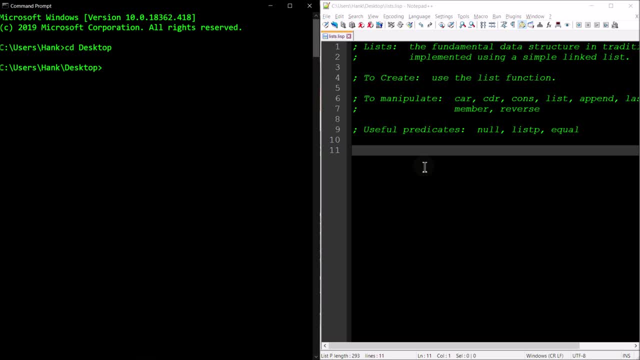 other lists right. whatever you can think of, you can put inside of a list, right? And so maybe the easiest way to create one is to use the Lisp function, right, So I'll go ahead and show you how to do that right? So if I want to create 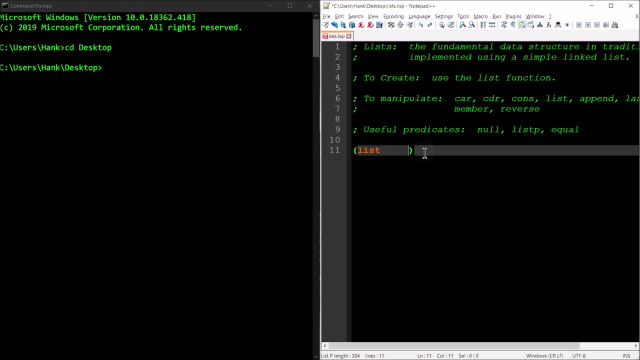 a list Lisp function and then everything after the list function. all the arguments are just gonna be whatever you want to put there as well. right, So I'm going to wait a momentations inside that list. right, so I could specify that I want a, B, C, 1, 2, 3 to be. 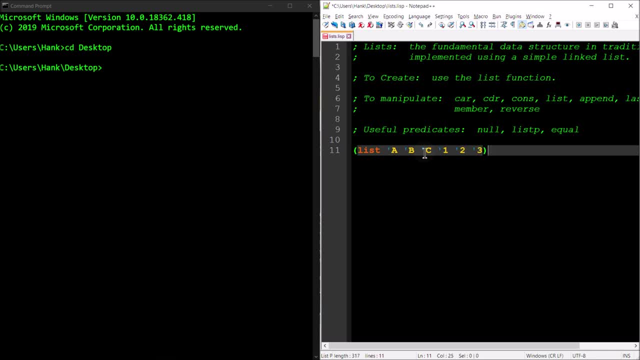 part of my list, right, and if I do that, then you're gonna see that the list is gonna get created, right. okay, now the pile is just fine, but what was there to show you? nothing, really right. so let's go ahead and assign this, or we'll just. 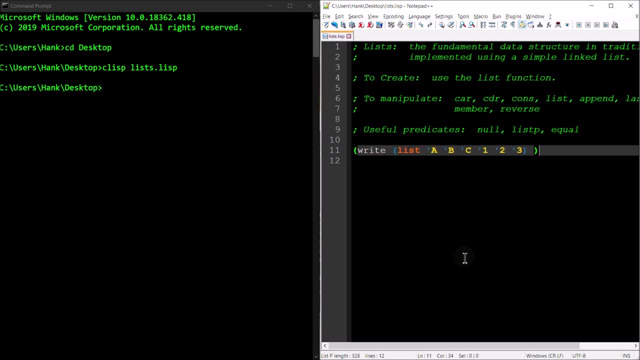 pass it straight to the right function. how about that? so we can see the results of that list getting created. all right, so there you go. so you see the ABC. one, two, three, four, five, six, seven, eight, nine, ten, nine, twenty-two, twenty-two, twenty-two, three. that created my list. now, if I wanted to actually be able to manipulate, 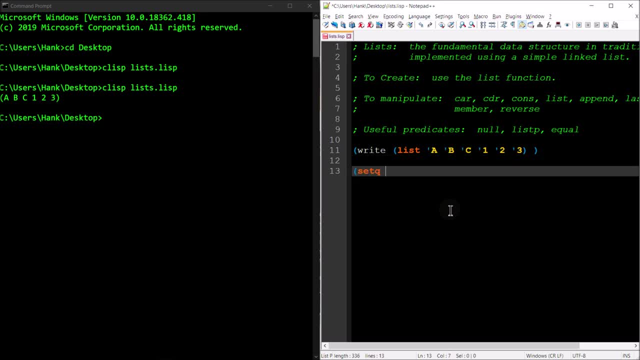 it in some way, then it might be useful to actually assign it to a variable, right? so I'll name this variable. you know, dog or something, right, it doesn't matter, I can name whatever I want, and we have some more kind of thing here, okay, and then i'll write out the dog. 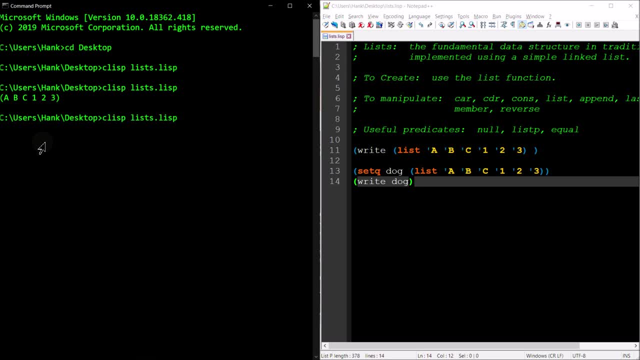 okay, so you should see that list get created a couple times. there we go, okay, um, and then you can also, um, create a list. you don't even necessarily need to use the list function. um, i could do something, uh like this. i could say: well, set q, cat, and then i can. 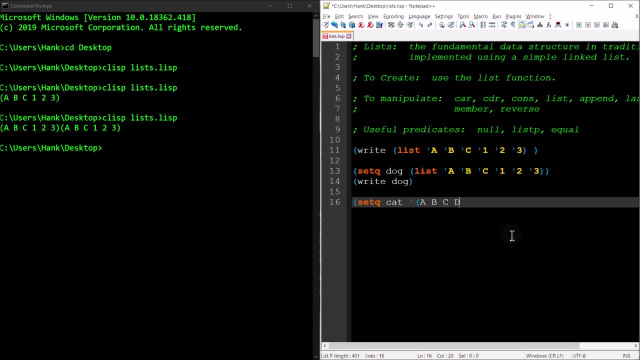 create a list right by um, just using the apostrophe here and then typing out what i actually want the list to look like, right, and so then i could write out that list. okay, so let's run it one more time, right? so there's my new list. so three different lists here. 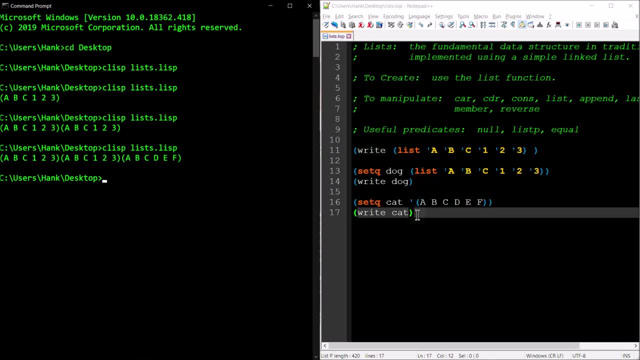 um, you know, made a couple different ways, right. so you know now. lists can have a mix of different types of lists. lists can have a mix of different types of lists. lists can have a mix of whatever you want to put inside them. whatever you want to put inside them. 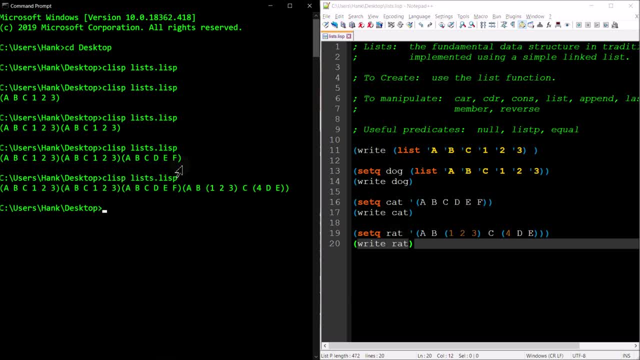 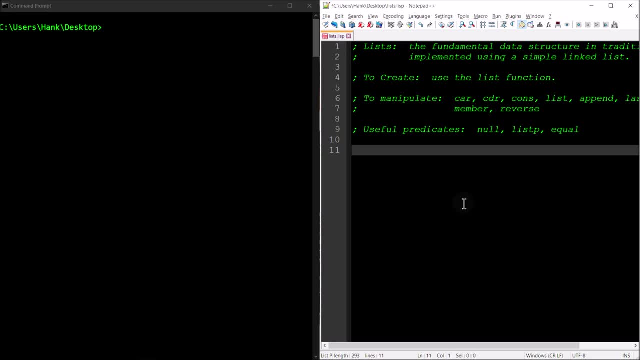 Okay So let's go ahead and run that. Okay, So you can see lots of different ways that we can create lists. Okay So, how can we manipulate lists, right? So let me just create a really simple non-nested list, right? 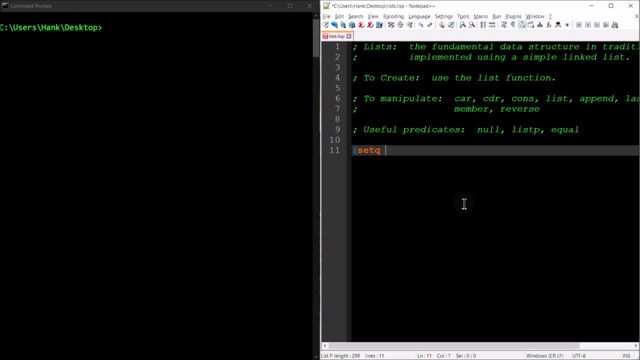 Okay, So I'll create a variable, I'll just call it cat And I'll use the list function to create the list And I'll just assign it. you know, just some simple characters here, just so we have something to display, Okay, And or to work with. I should say: 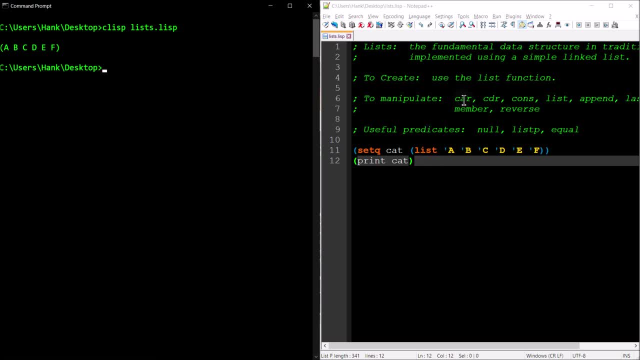 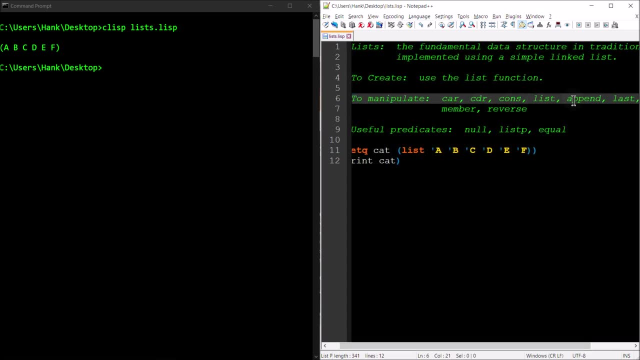 Okay, And let's run it. So there's our list. Okay, So let's run it. So there's our list. Now I want to go through these different functions for manipulating, right? So we've got car cutter cons list. Well, I already showed you list, right? We use that to create functions, So I suppose I could get rid of this guy from here, But append last member and reverse, right? So how about we go through and play around with these guys in no particular order? 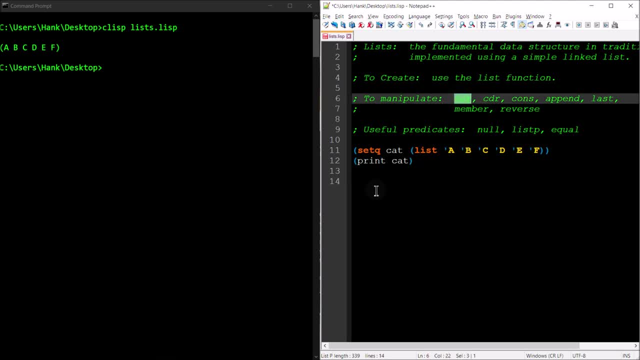 Okay, So let's go ahead and run it. The car function here, right, If I pass to the car function a list, right? So, for example, the list that is defined with cat, right, And I print that thing out. So what car does is it peels off a copy of the first item in the list, right? So you can see that the list is defined with cat. 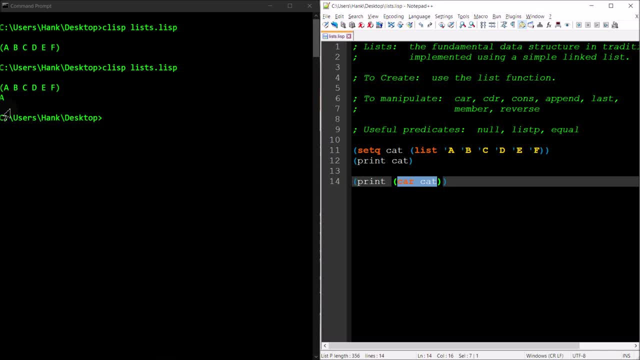 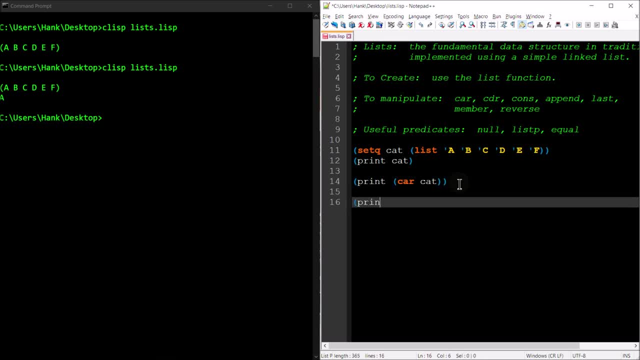 Okay, Okay, Okay, Okay. Okay, print out cat again. you'll see that the original list hasn't changed right. so it just peels off the first item in the list but doesn't remove it, right, it just returns a copy of it, okay, so that's. 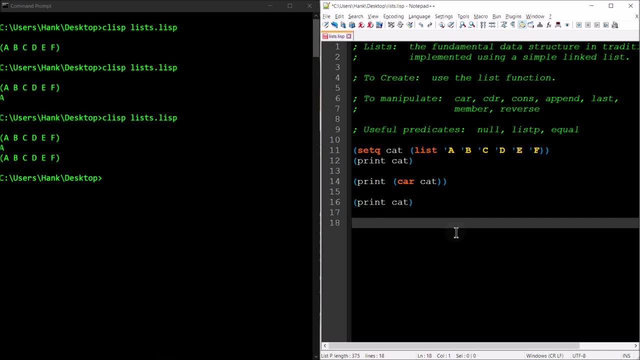 what car does? now? what about cutter cdr? right? so what cdr does is that returns a list. that is everything but the first item in the list, right? so let me just show you. so cutter cat, right. and this guy also is non-destructive, right? so the original list is going to remain unchanged, okay? 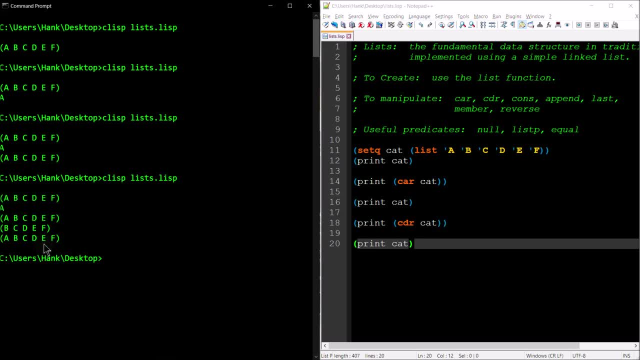 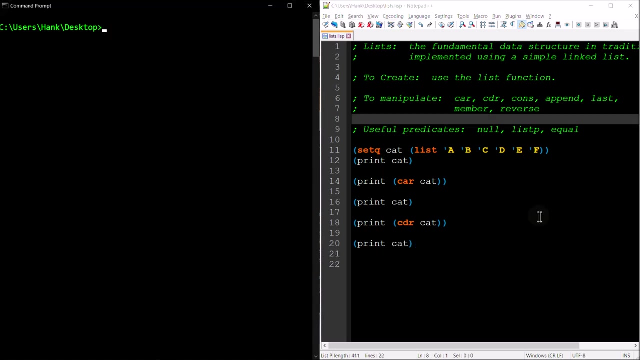 so, okay. so, if we can see right here, BCD, EF, that's the remaining portion of you the list, right? So that's line 18, the results of line 18.. And you can see that the original list that I assigned to cat has remained unchanged. Okay, so let's talk about cons And the cons. 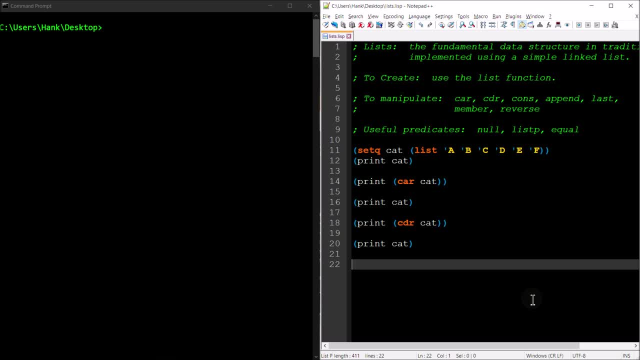 function can be used to create a new list that is the combination of two existing things, right? So let me give you an example here. So if I wanted to combine the list A, B, C, D, E, F, I want to get. 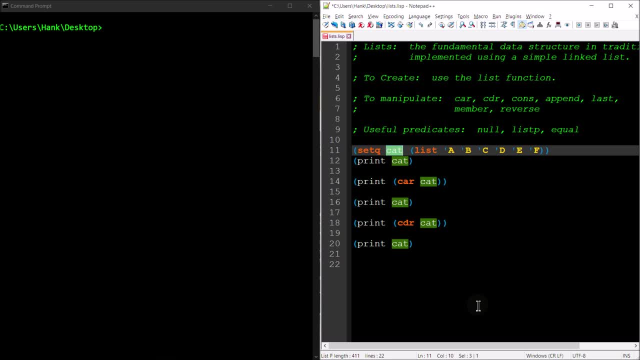 that cat list And then I wanted to make that list be the first item in a new list And I wanted to put say G as a second item in that new list. then I could do something like this, right? So I could. 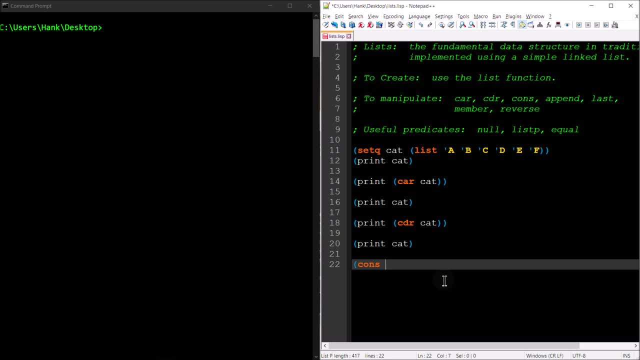 say the cons, and I would take the name of the first item that I want to have in the list- in this case it's itself an entire list- And then I would then use cons again and specify the name of the thing that I want to be. 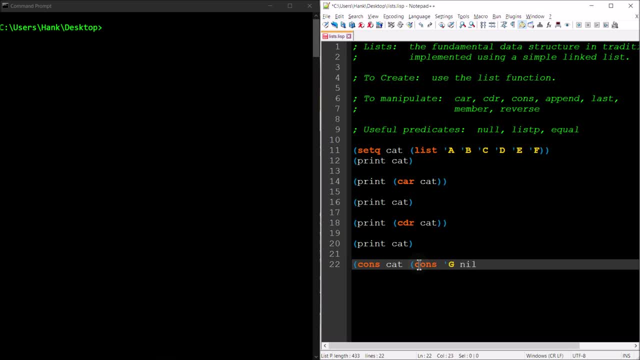 becoming the second part of the list, And then I would add new here, right? So what this is going to do is this is going to create a new list where the cat list is the first element And then I would say G is the second item, right? So I'll just go ahead and print that and show you what it looks. 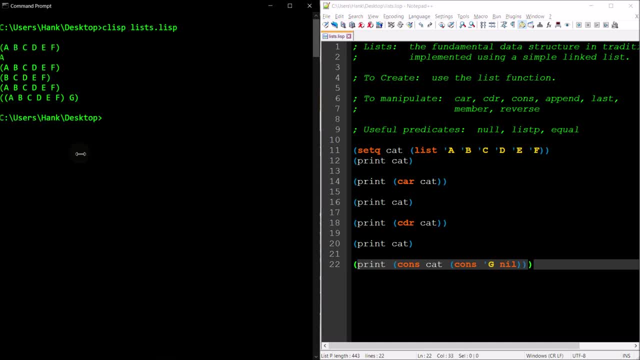 like: Okay, so there you go on your bottom line. So you've got a new list. A, B, C, D, E, F list is the first item and then G is the second item. Now, this is kind of a convoluted way of making. 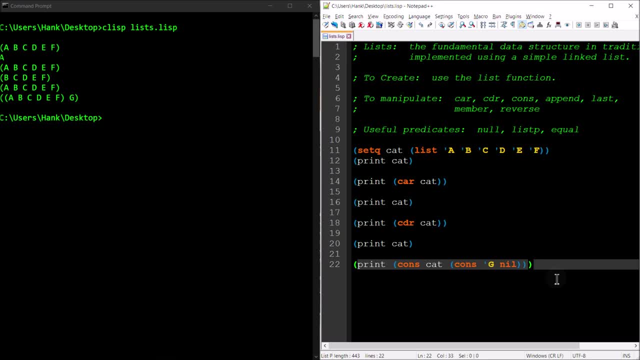 new lists. It would be a little bit, a lot easier just to do this with a new list. So I'm going to go ahead and print that out And then I'm going to go ahead and do this with the list function. So if we were to do something like this, say, list cat G: right, 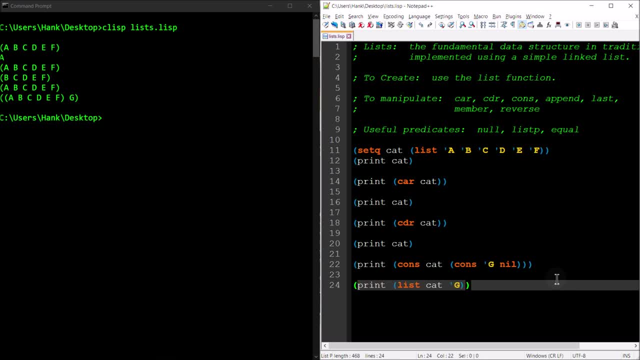 and you can see that that's going to be a lot easier to do. So let me go ahead and run this So see, we get the exact same result And we don't have this nested recursive kind of a structure going on here, But without that list function. and you wanted to create a new list, say containing 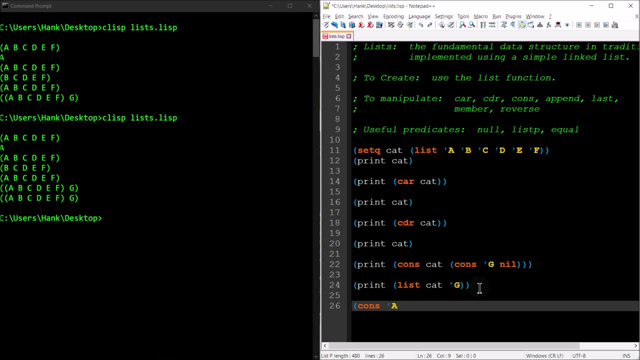 ABC. you'd have to do something along the lines of this: you'd say cons of A, and then you'd say cons of B, And then you'd say, I mean, it just gets gross. Then you'd say cons of C, and then you have nil. 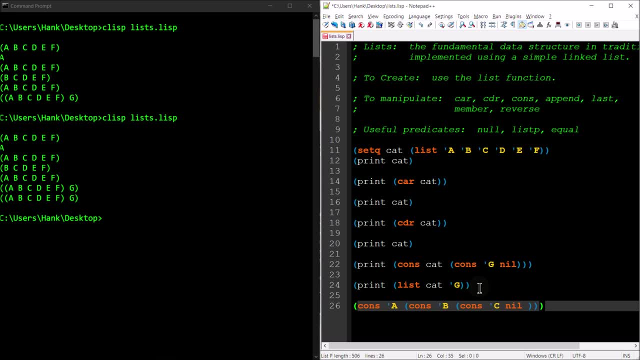 there and then you close this whole thing off And then I'll just pass this straight to the print function, So you can. so you can see what it would look like. So it's kind of gross creating new lists that way they can see the ABC right. So list function. 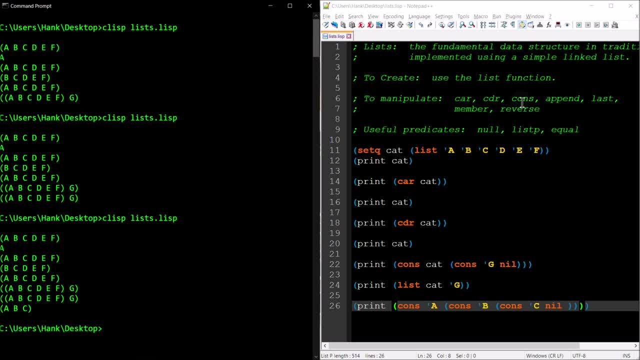 is definitely a lot easier. The main use for cons is really to create these dot pair structures within Lisp, But you know cons works this way as well. Okay, so let me show you how the pen function works. The pen function. 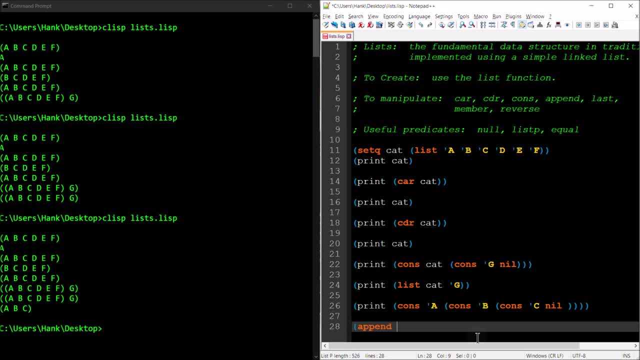 you know you're gonna type that, append up there, and then you can string together a bunch of lists and as arguments and the result will be a new giant list, right? So I could do something like this. I could say: well, we'll take A and B and then we'll append to that C and D, and then we'll. 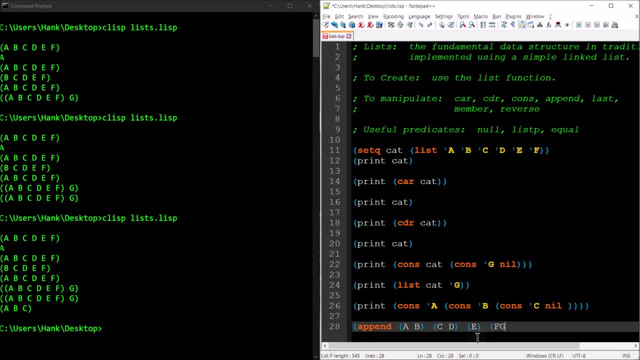 append to that E and then we'll append to that F, G, H, right, And I'll just send that that new list straight to the print function so you can see what it would look like, And I'll go ahead and run this thing here And you can see. oh, I forgot my single quotes here. 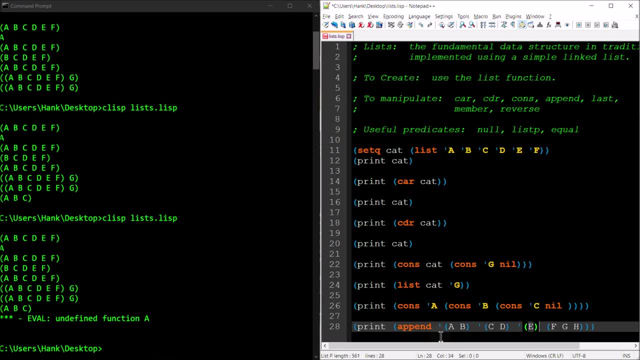 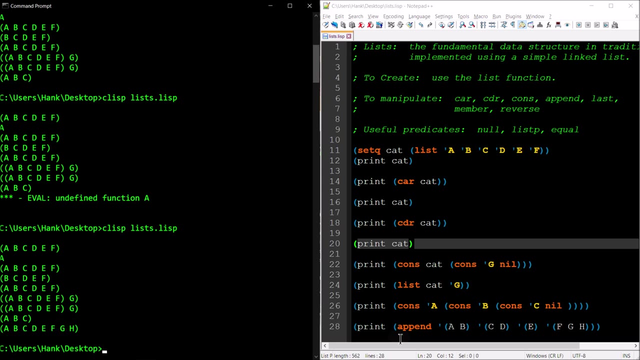 right, Because, remember, Lisp tries to evaluate even items in the list. if you want to create a new list with them, right? So let me go ahead and fix that, run it again, And so now you can see there's our A, B, C, D, E, F, G, H, right. So that created a brand new list. 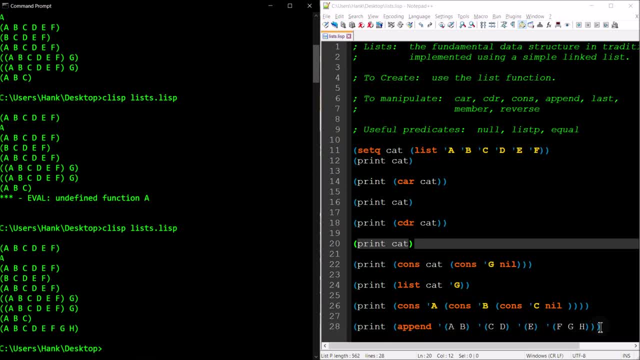 for me that is concatenating all of these other lists, okay, So you know, you could imagine that it'd be really easy to combine car cutter, append in different combinations to get you, you know, whatever list that you need. okay, So another example of this, you know. 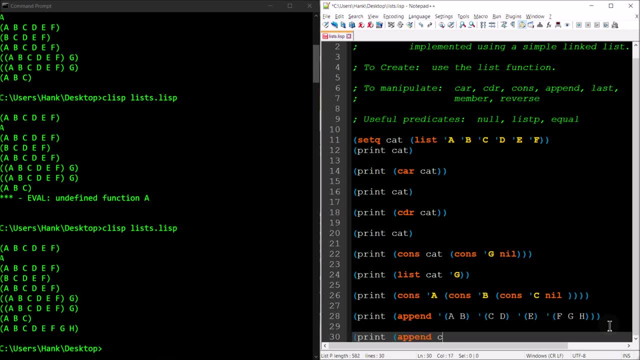 let's go ahead and take our cat list and then we'll append to cat G And then I'll just print it straight out so you can see what it looks like. okay, So you can see the last line. there there's the result of us appending G to our cat list. now 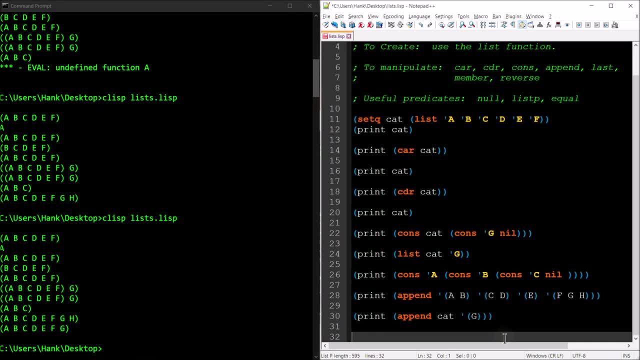 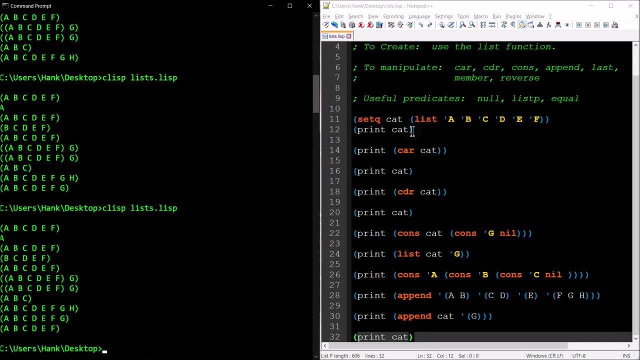 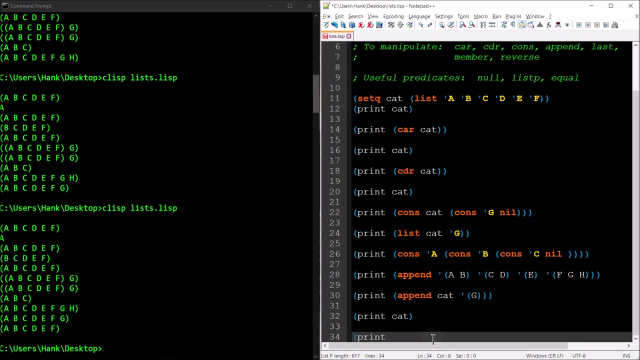 Now that creates a brand new list, right? If I just print cat out again, you'll see that the original list that I assigned to cat unchanged. Okay. so what about last? Okay, well, last is kind of like the opposite of car, right? So how about we just do? 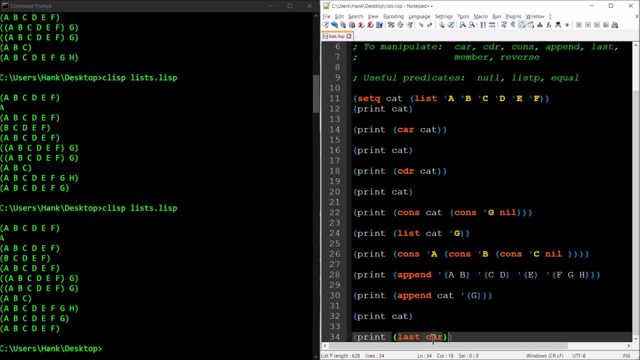 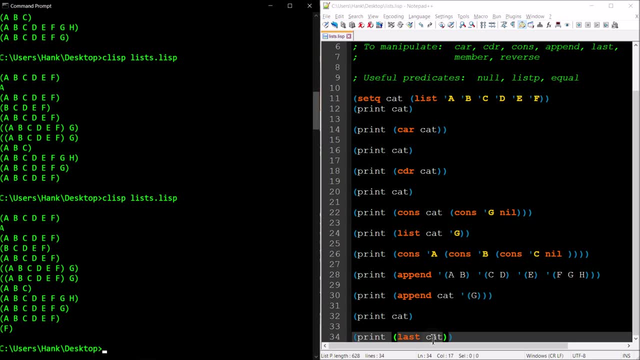 print out the last of car and we'll see or not. car sorry cat, our cat list and we'll see what we get. Okay, so you can see there's a F right now. Last is not exactly like car, because remember what car does is it returns a copy of the first. 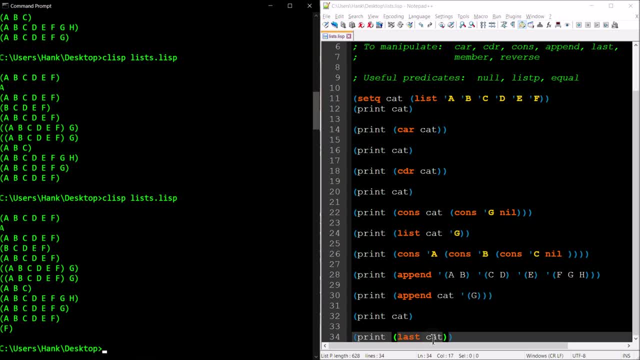 element of the list, right? So what last does here is it returns a list that contains the last item in the list. okay, If I wanted to do something more like with what car was doing, but for the end of the list I could combine car and last cat, right? And so what's going to happen? Well, 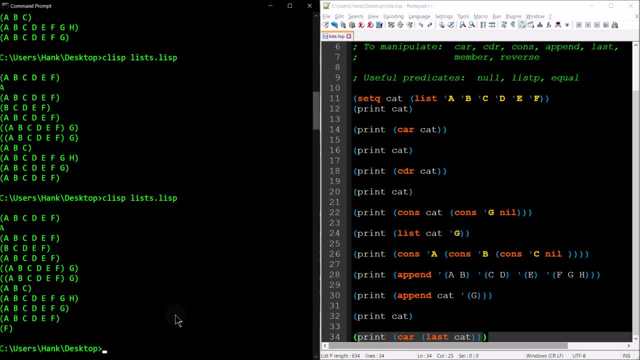 remember, car just peels off a copy of the first item in the list, right? So now you can see there's just a regular f, right? so car last cat is kind of like, um, the opposite of car cat, right, you just got to combine. 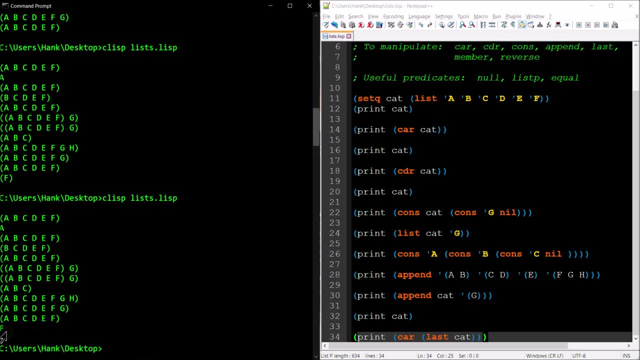 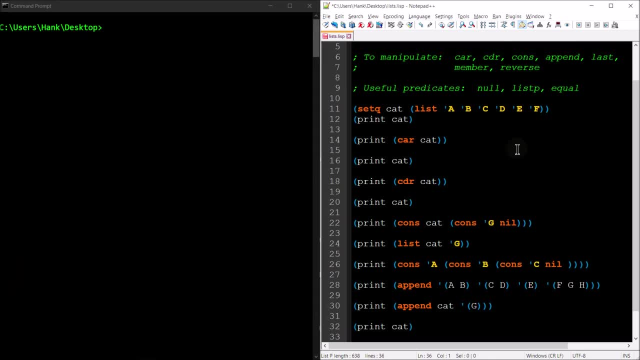 those two things together to be able to extract the first or, excuse me, the last item from an existing list. okay, so let's take a look at the member function. member function is going to take two arguments and the second argument is going to be list, and then the first argument, if it is a 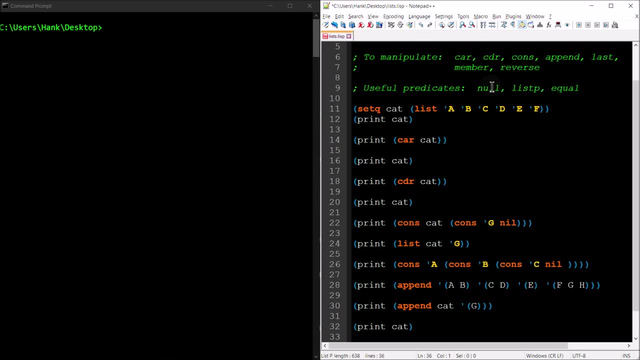 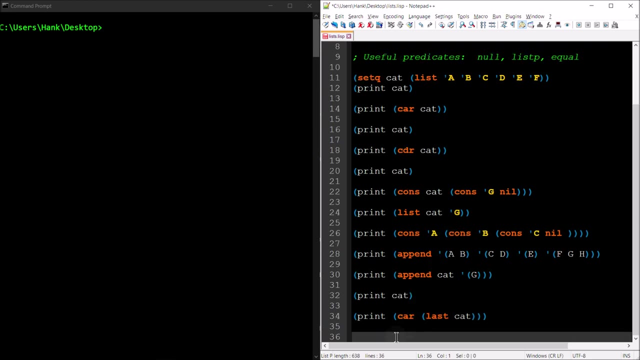 member of the list specified in the second argument, then this is going to create a new list or return a new list. that is everything. um, after the first argument, right? so let's give this a try with cat. so, uh, we'll do something like this, right? so remember. and then let's say that i'm going to 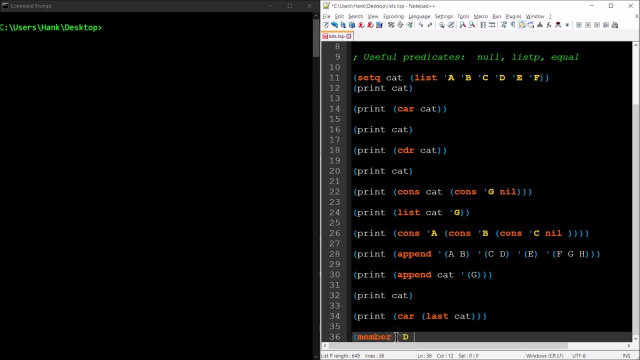 look for um d in the second list. on the second list, i have that assigned you verbal named cat, right? so I'll just print out the results of it and we'll see what we, what we have right. so there's the last line, def, right? why did? 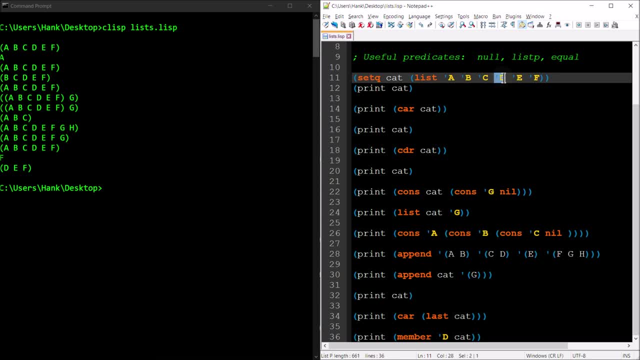 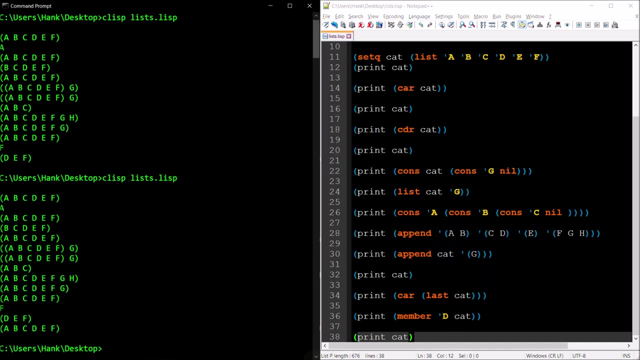 we get that well, because there's D. right, there's the first argument. and so we got the def out of this thing now again non-destructive. if I print cat out again afterwards, you're gonna see that the original list still unchanged. and keep in mind these functions I'm showing you. you know what they're doing is they're? 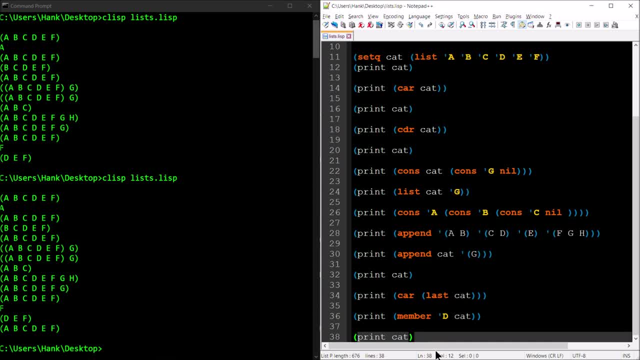 returning a list or, in the case of car single value, which you can then use later on for for later processing. so, for example, you know what, if I wanted to pull out that def and use it for something else, maybe I'll call it dog um and I'll say what number D cat right, and then I can print out the dog right and 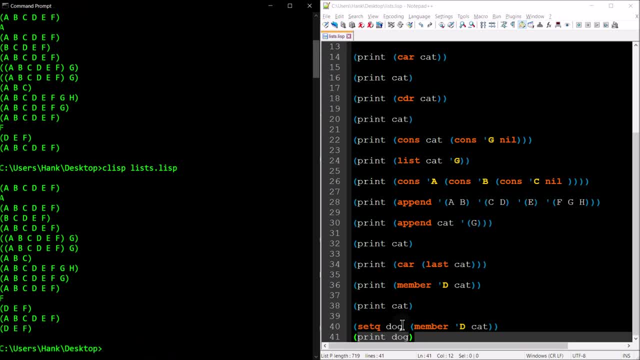 let's see what this, what that looks like, right, so you can see with the output right, I printed out cat on line 38. there's the original list, unchanged right, and then I created a new list that is made up of everything from D through the end that belongs to cat, and so I called that. 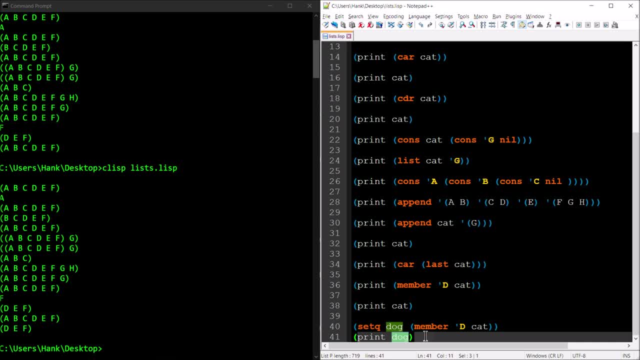 list dog, and then I printed out the dog right. so the last function that I want to show you here- and then I'll show you a couple of predicates and how those work- is going to be a reverse. so what does reverse do? well, all reverse does is: 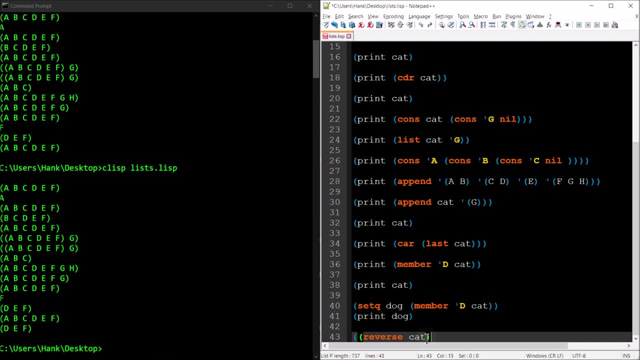 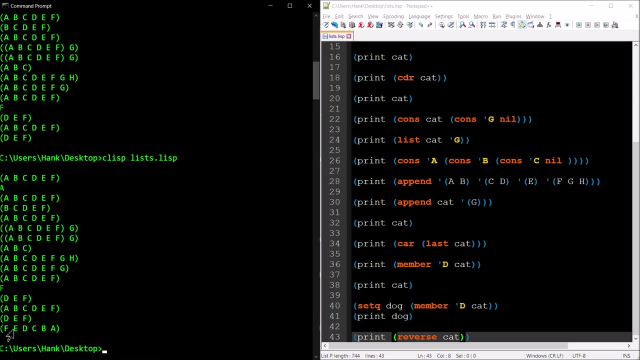 gives you a new list that's in the reverse order, so I'll just go ahead and print the reverse of cat to the screen for you and show you what that looks like. okay, so there you go. F, B, D, C, B, A. now, if I wanted to pull off a copy of the F item, another way that I 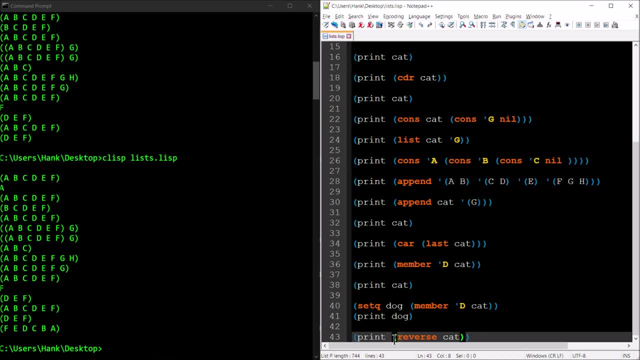 could have done it right. I showed you combining car last. well, I could combine color in reverse and have the same effect, right. so there you go, okay. so the last thing I want to show you is the. you know the key, so I'm going to do this and 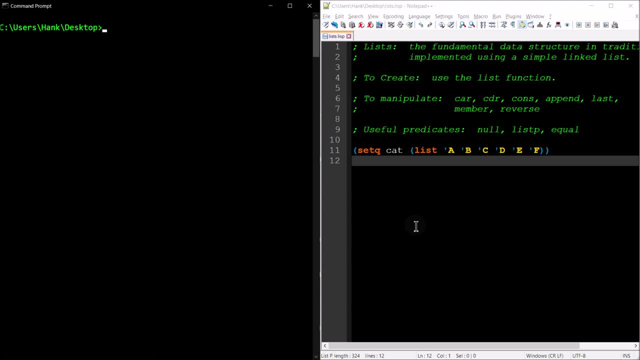 are a few useful predicates that could be helpful when dealing with lists. Those will be null, list p and equal. Predicate is like a Boolean function, right? What you do with predicates is you feed them some arguments and they return true, or 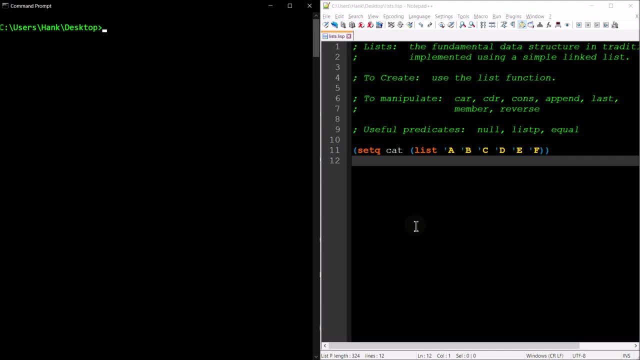 nil, t or nil right. So t is true, nil is equivalent to null or false in Lisp, right. So first one that I'll show you is null, And null takes as an argument, can take as an argument a list, right? So I'll give it cat and then I'll just print out. 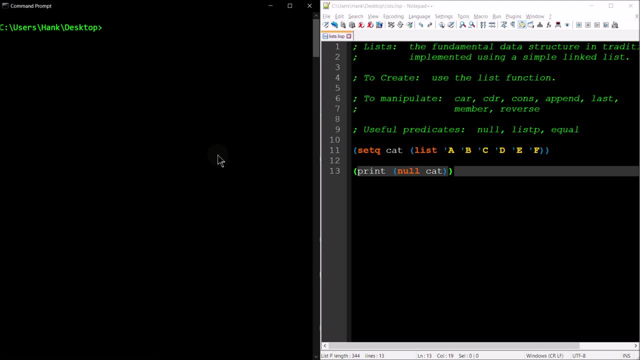 what it returned, right? So what that's gonna? you'll see, it's gonna show us nil, because why? Cat is not empty, right, There's actually something in that list, right? But if instead, you know, I gave it a list and this is a list, right here? 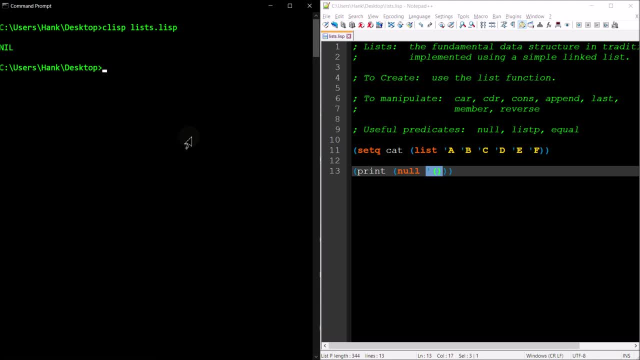 with nothing in it, then that's gonna evaluate to true right, Because this list is null. There's nothing in it, right? So I'll give you. I'll leave both versions up here so you can compare them side by side. 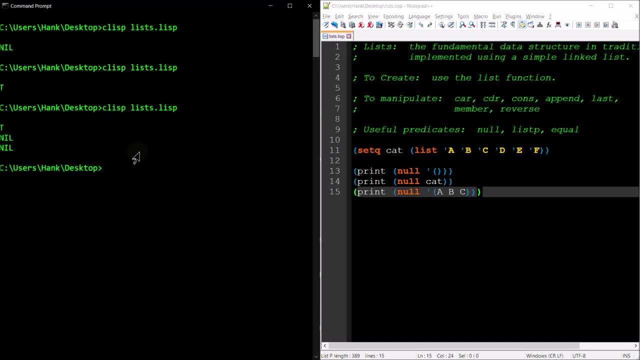 So that null function can be useful as or for the base case of recursive functions. You know, if you're recursively going through a list and passing back smaller and smaller versions of the list until eventually there's nothing left inside the list, well then null could be useful for for getting you out. okay now. 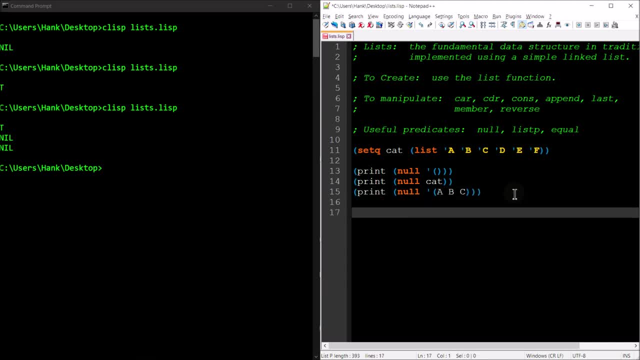 of your recursion. Now, list P is going to return, true, if the thing that you, the argument that you pass it is actually a list, right? So cat is a list, so it's gonna return t, right? So you're gonna see that here in a second. So there you go. Now what if I were to pass it? 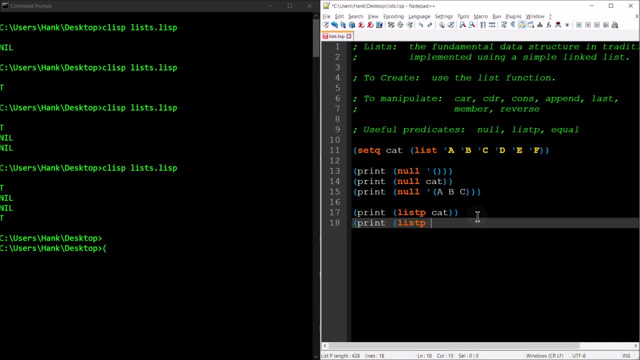 something that wasn't a list right, Like maybe 8, right? What's gonna happen? Right, nil, Why? Because 8's not a list, right? Okay, and then finally equals, Or equal. Now, the equal predicate is what you'd want to use if you want to see if. 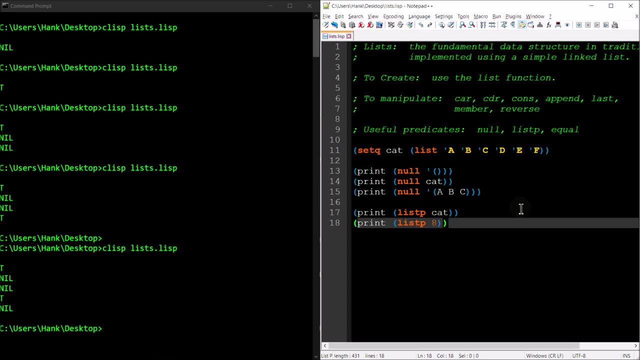 two lists are structurally the same right, So this is different than trying to determine if 7 and 4 are equal or not, right? I mean this is lists themselves in Lisp are objects, and so a simple arithmetic equals isn't going to do it. 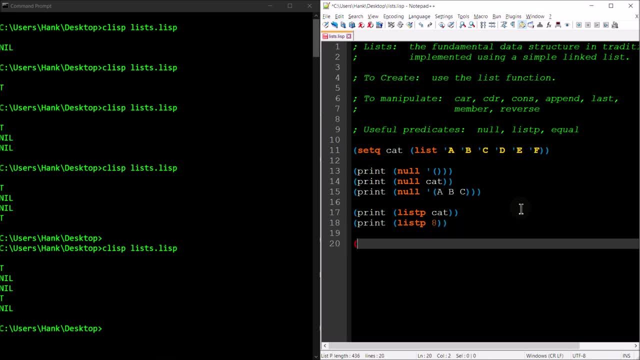 right. So we need to have something a little more involved. So that's what the equal function does. So we'll take two arguments right, And so maybe I've got the list a, b, c and the list a b c right. So this is gonna evaluate the true, which you'll see when I print it. 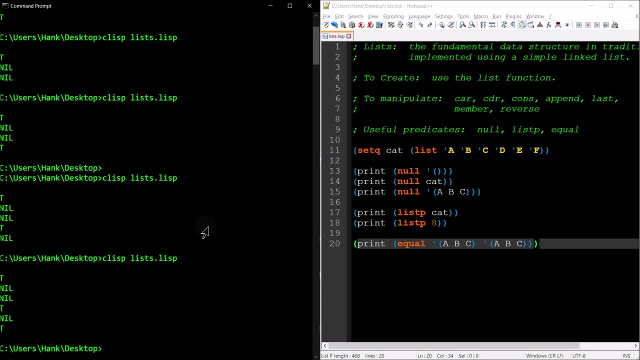 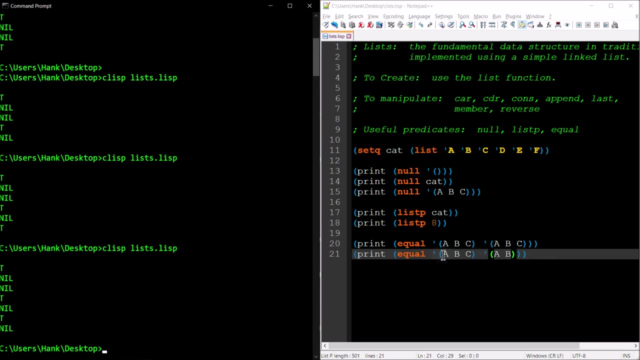 out because the lists are the same, right. So there's your t for true. If they were different, so let's say we make this just a b and that's gonna return nil. And you know, I put in some lists here using this apostrophe operator here, but you know.